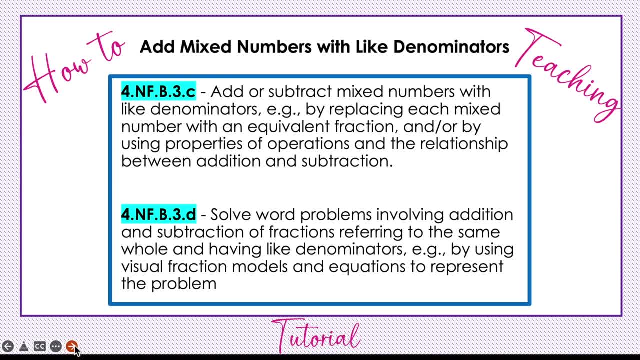 When working with mixed numbers, using word problems provides context for students and allows for the concept to be more relatable. In this tutorial, we'll look at specifically adding mixed numbers with like denominators, using properties of operations and solving word problems involving addition of fractions referring to the same whole. 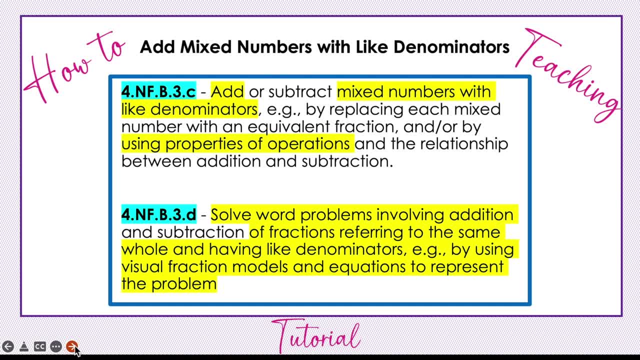 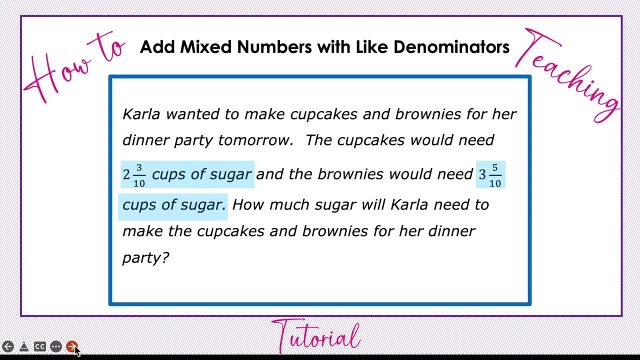 and having like denominators, by using visual fraction models and equations to represent the problem. So, looking more closely at this problem, we know that Carla needs to join the cups of sugar that she needs for the cupcakes and the cups of sugar that she needs for the brownies. 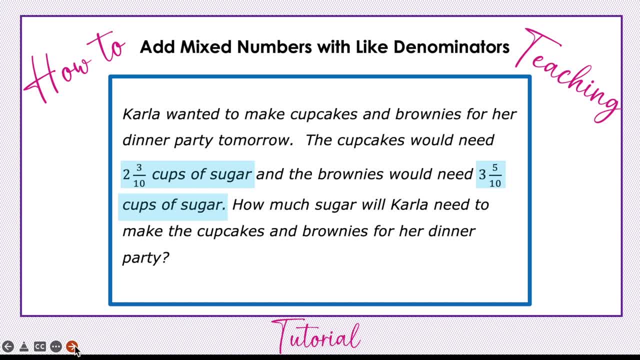 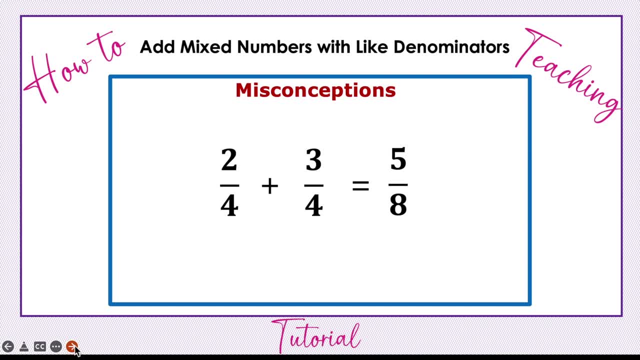 So we're gonna take two and three tenths cups of sugar and add that with three and five tenths cups of sugar. Before we start, let's look at a common misconception that students might have when they are adding mixed numbers. One misconception students may have: 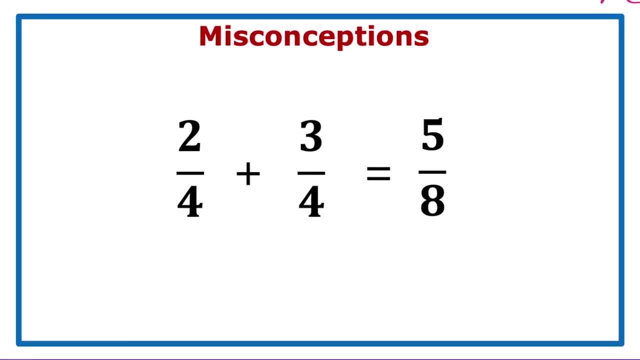 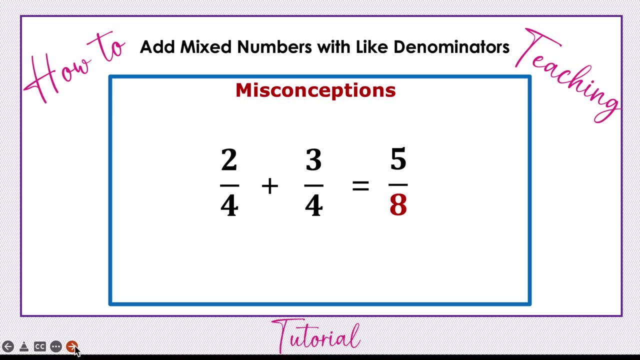 is that after adding the numerators together, they think they will need to add the denominators together as well. This will show you that your students don't really have a full understanding of what a fraction is. In the book The Common Core Mathematics Companion. 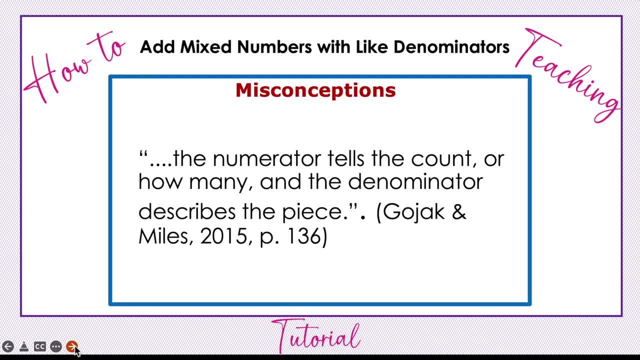 The Standards Decoded by Gojek and Miles. they emphasize the meaning of the numerator and the denominator when referring to misconceptions with adding fractions. The numerator tells the count or how many, and the denominator describes the piece. Many students and some adults don't fully understand. 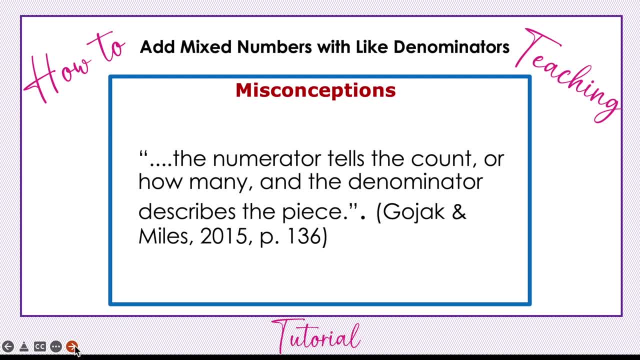 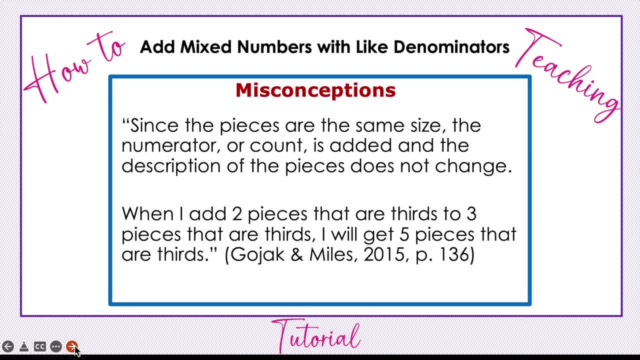 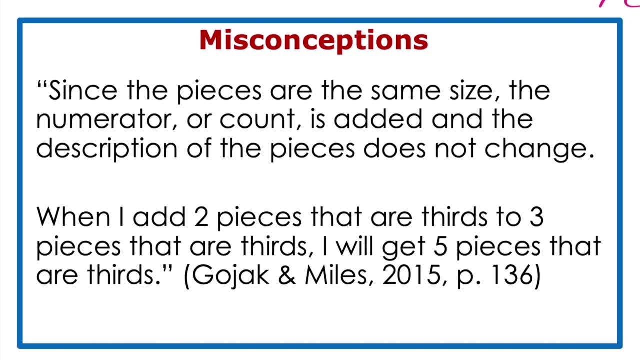 that the denominator in these cases is a descriptive word that describes the size of the pieces, not the number of pieces. We add amounts, not descriptions. They give a great example in the book. Pieces are the same size. the numerator or count is added. 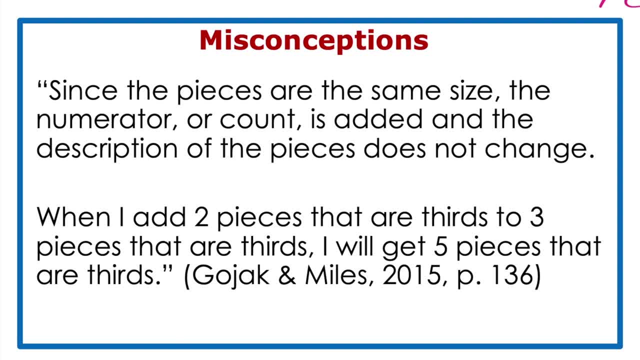 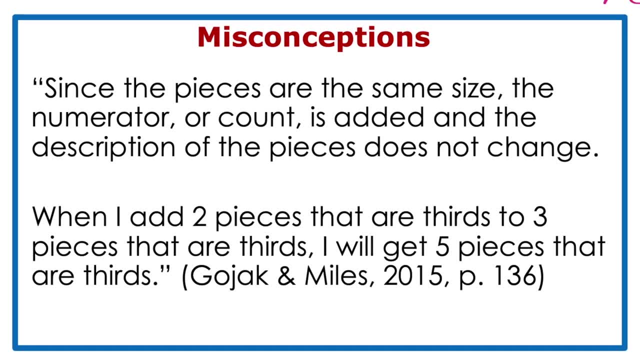 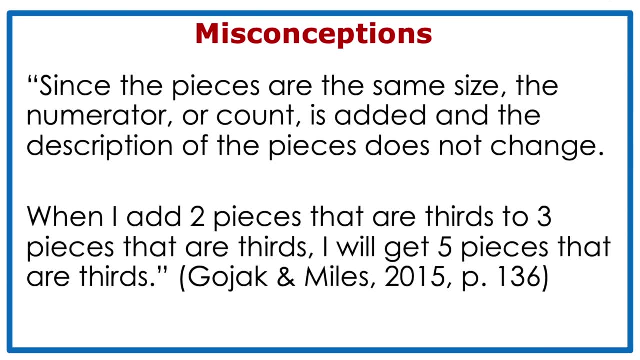 and the description of the pieces does not change. When I add two pieces that are thirds to three pieces that are thirds, I will get five pieces that are thirds. Thinking about it this way can cause you to focus on the denominator as a description and not just a number or digit. 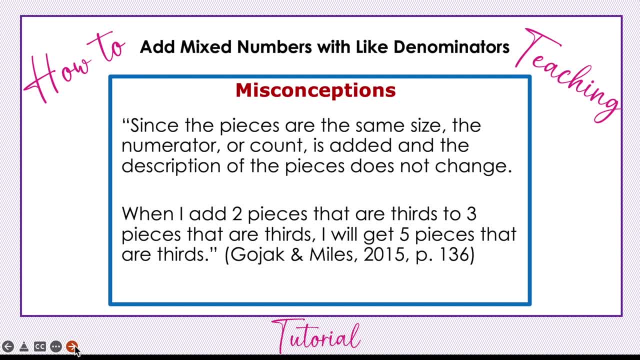 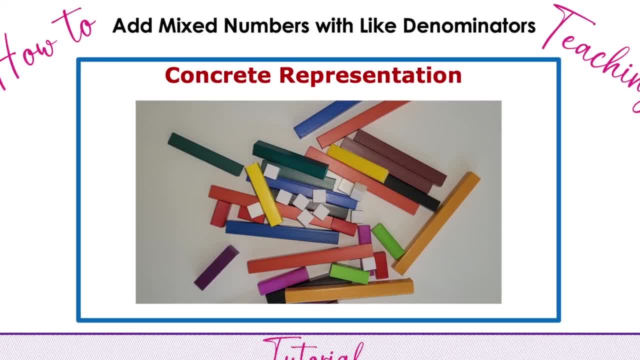 I highly suggest thinking about possible student misconceptions before teaching a specific lesson to students, so you can plan for what they may possibly do. Let's keep learning by looking at a concrete model of our problem. For this example, I'm going to use Cuisinart rods. 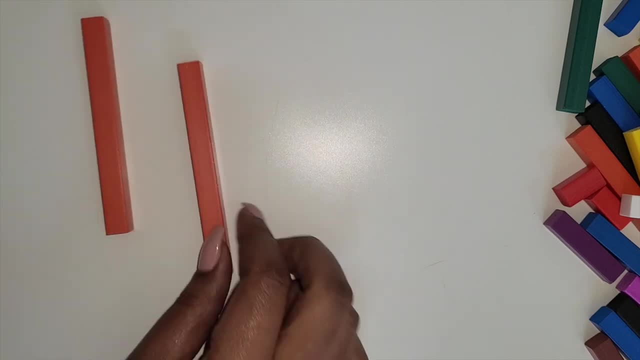 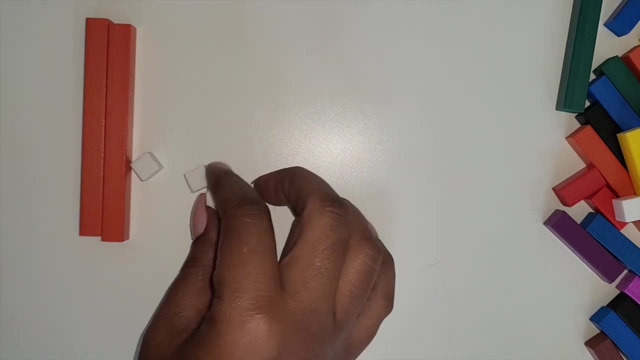 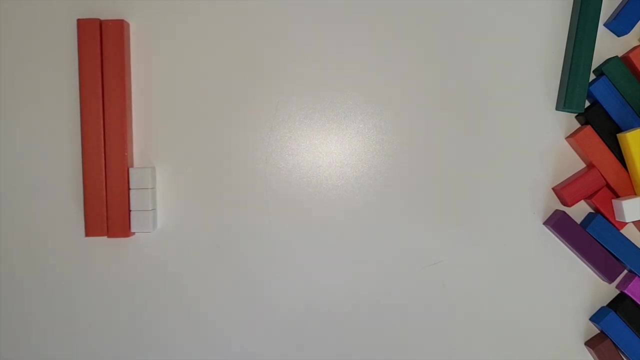 to represent both mixed numbers. The orange rods will represent the holes and the white rods will represent the 10th size pieces. So we're going to show our first mixed number: two holes and three 10th size pieces, or three 10ths. 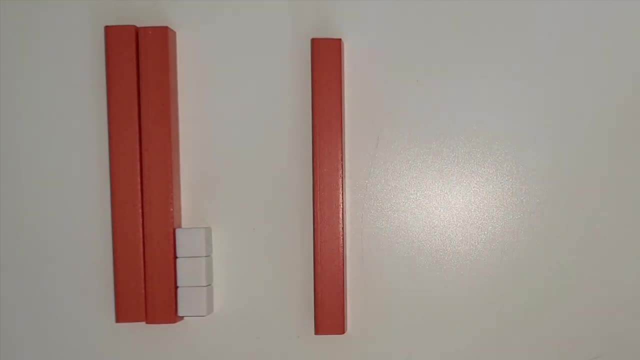 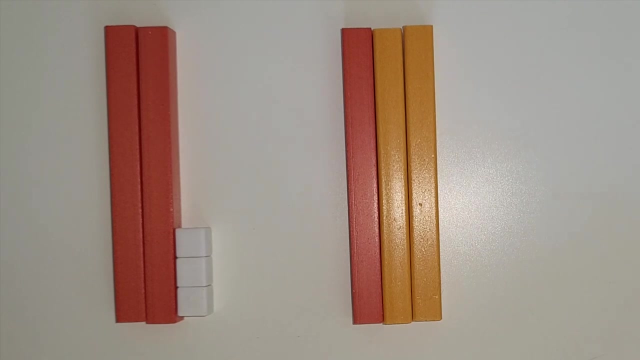 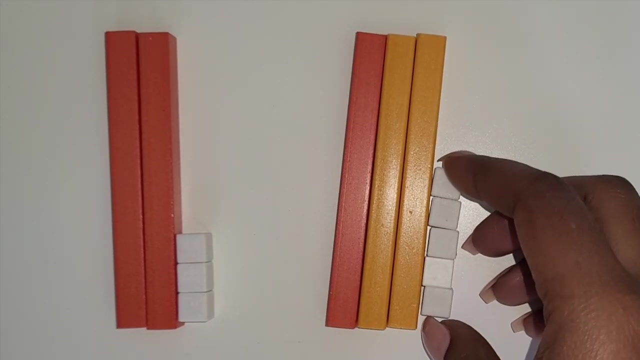 The white rods are 10th size pieces in this scenario, because it takes 10 of them to equal one hole. Next, we're going to join that together with or add on our second mixed number: three holes and five 10th size pieces, or five 10ths. 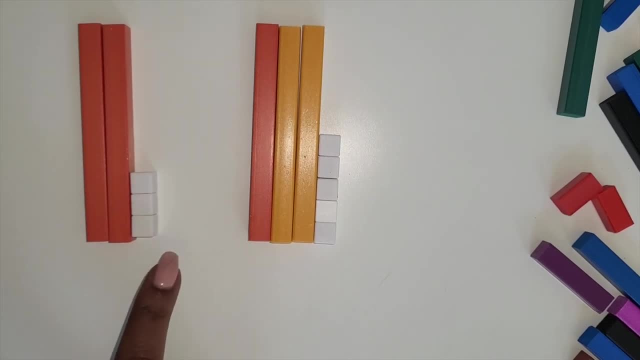 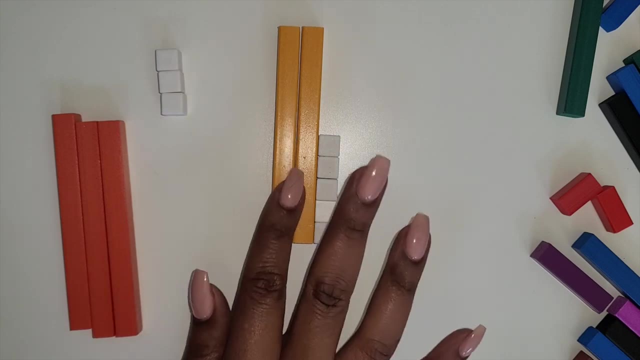 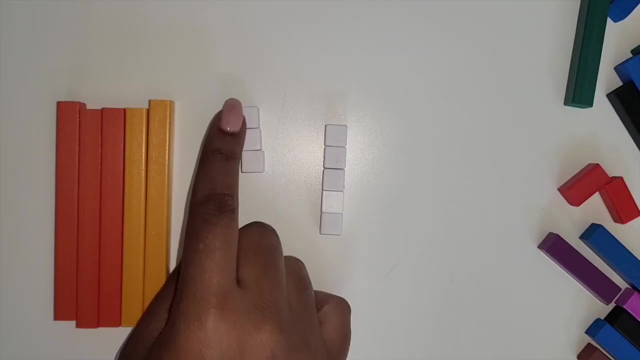 Starting with the whole numbers. when it comes to adding mixed numbers, you can first join all of the whole numbers together. Two plus three equals five. There are five holes in all. Now let's combine the three 10ths with the five 10ths. 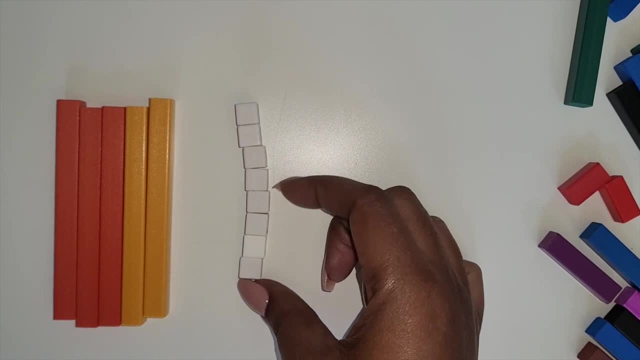 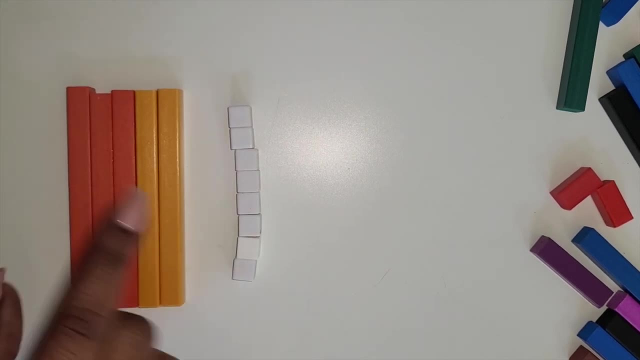 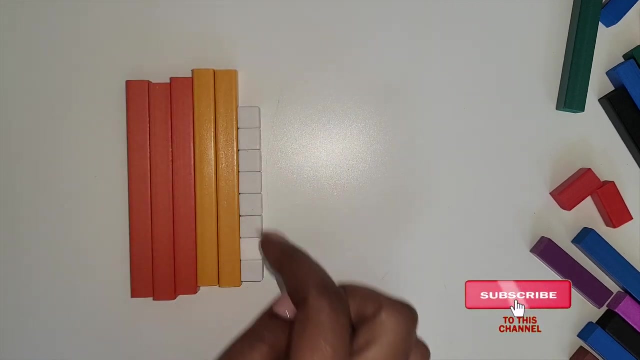 Three 10th size pieces plus five 10th size pieces equals eight 10th size pieces or eight 10ths. Last, let's join the five holes together with the eight 10ths. Five holes plus eight 10ths equals five and eight 10ths. 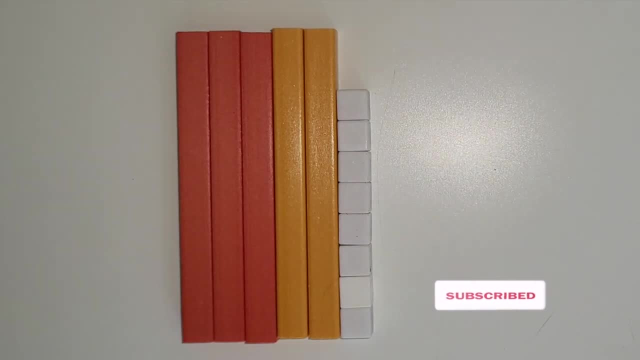 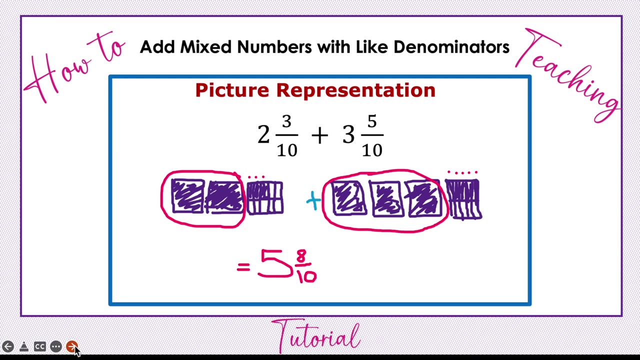 So, returning to the word problem, Carla will need five and eight 10ths cups of sugar. Once students are ready, move them along to drawing their own picture models to represent the actions that took place with the concrete model. This can be done on paper or a small whiteboard. 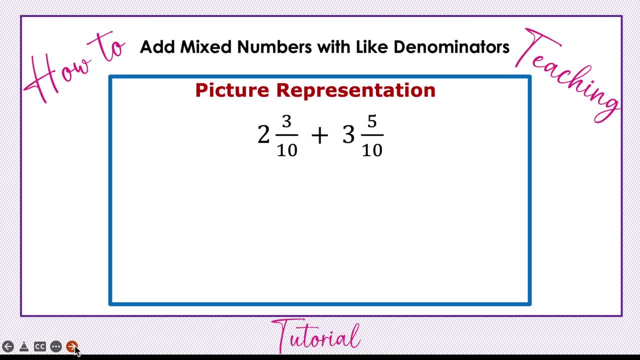 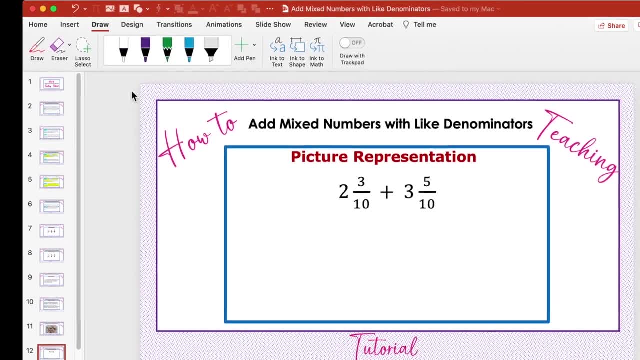 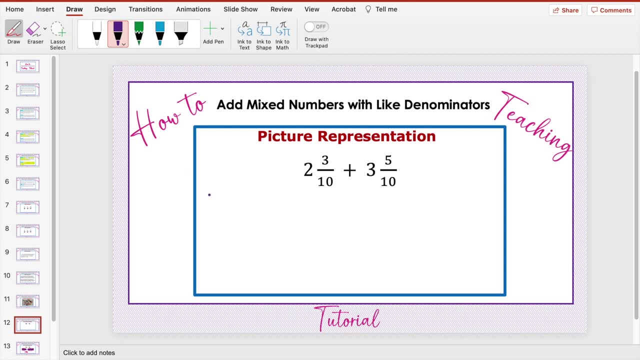 Here I am drawing it out digitally. for those who have students working remotely, I'm using the drawing tools in PowerPoint, but you can use any online program that has a whiteboard or a blank white space. Let's represent the two holes and a third hole that is partitioned into 10ths. 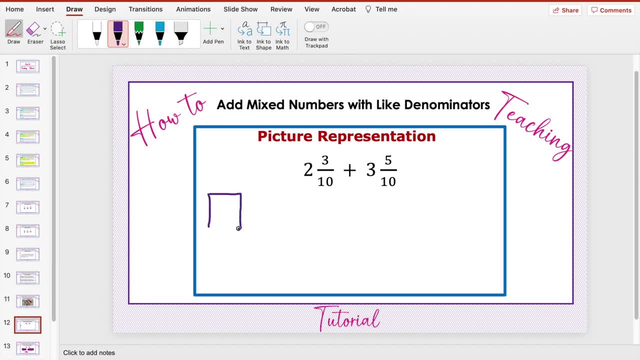 There is no specific model that has to be done. I find that it's typically easier to draw square or rectangle models than it is circular models. Whichever type of area models the students are exposed to more is the type of model that they are more likely to draw themselves. 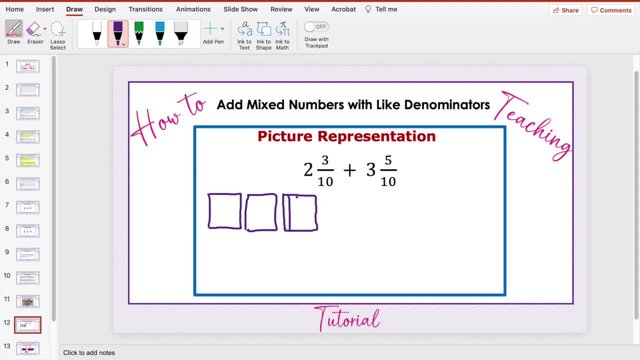 Remember to emphasize that each hole must be the same size. After drawing the two holes and shading them in, shade in three 10ths to represent the fraction part of the mixed number, Do the same with the second mixed number. Draw three holes and shade them in. 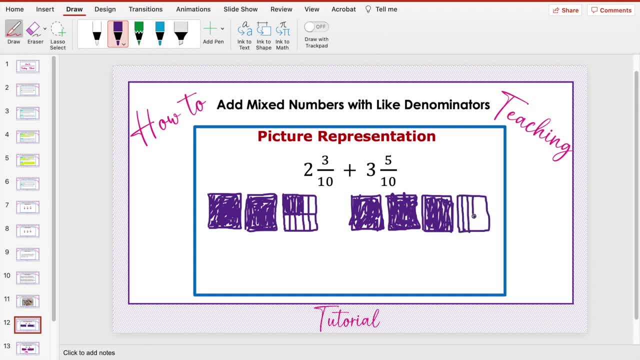 Draw a fourth hole to partition into 10 equal parts. The models drawn for the second mixed number should be the same as the first mixed number. Shade in five 10ths to represent the fraction part of the mixed number Circle. the picture of the holes in both mixed numbers. 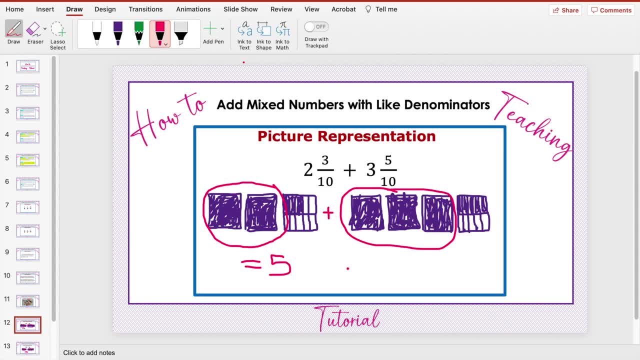 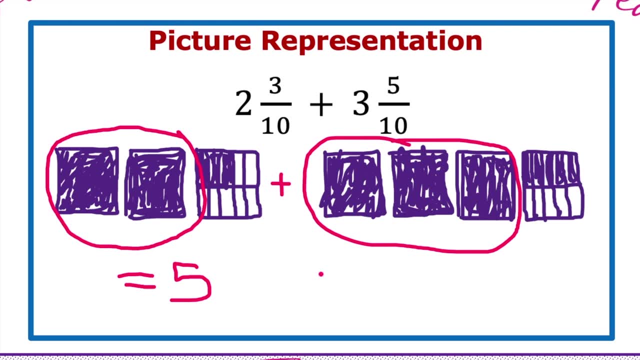 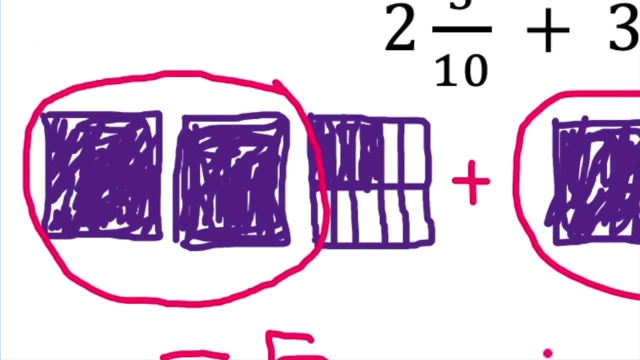 When joined together, two holes and three holes equals five holes. Now we can add the fractions together. This would be a great time to remind students, or better, ask them, if you are able to add the two fractions together. Are the parts of the holes the same size? 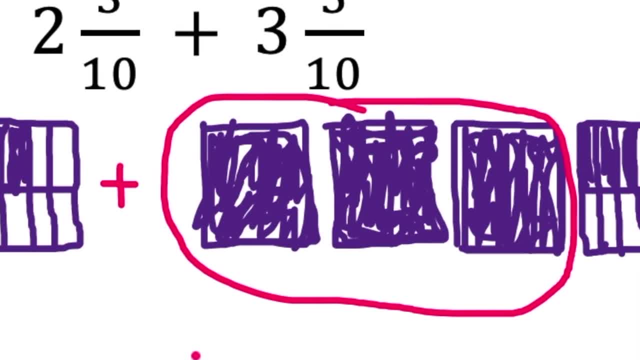 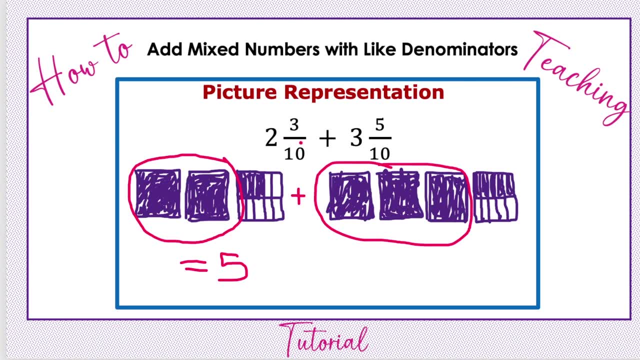 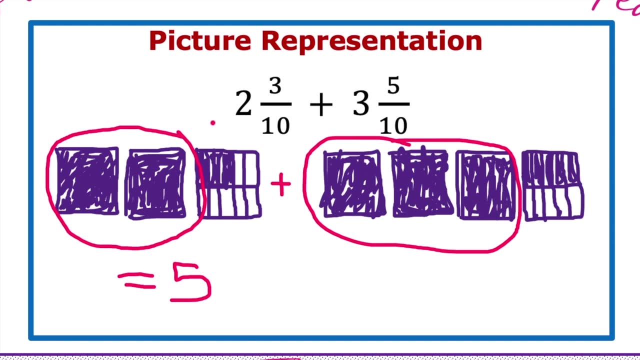 Some students may stare at the pieces and analyze if they were drawn exactly equal to each other. If this happens, refer to the fraction numerals or the denominators? Do both fractions have 10 size pieces? Yes, When we add three pieces, that are 10ths. 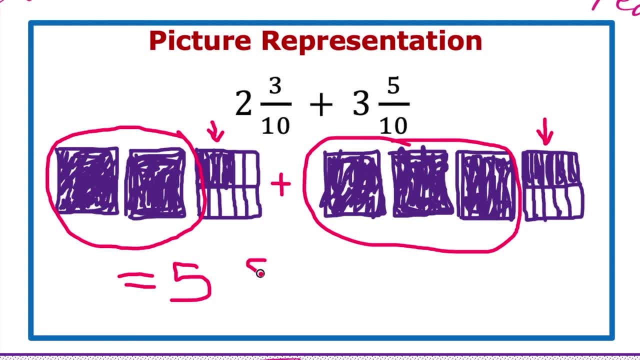 to five pieces that are 10ths. we now have eight pieces that are 10ths. We can also say eight 10ths. Don't forget about that whole number. When we add five whole pieces, we can also say eight 10ths. 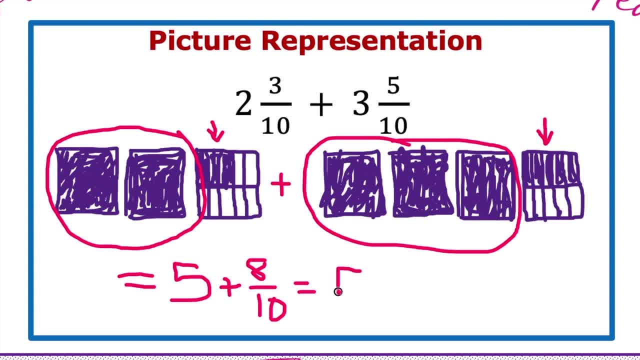 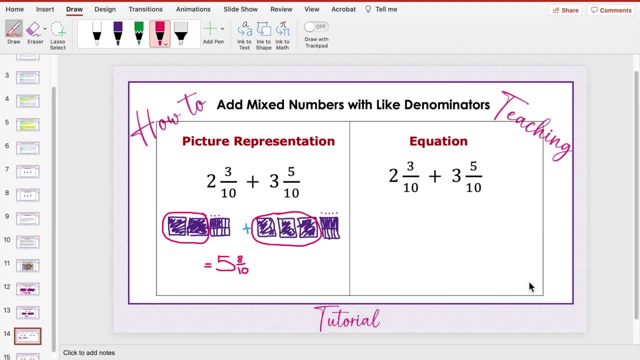 So if we add five holes to eight 10ths, we get five holes and eight 10ths, or five and eight 10ths. Now let's connect what solving this problem looks like visually to an equation We can see from the end of the picture model. 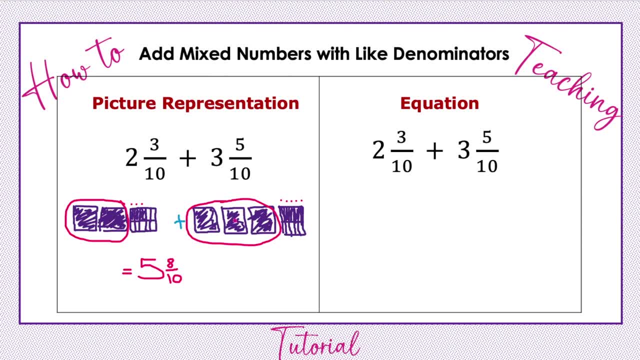 that we circled the two holes and the three holes With the equation. we can rewrite it with the two whole numbers next to each other and the two fractions next to each other: Two plus three plus three 10ths plus five 10ths. 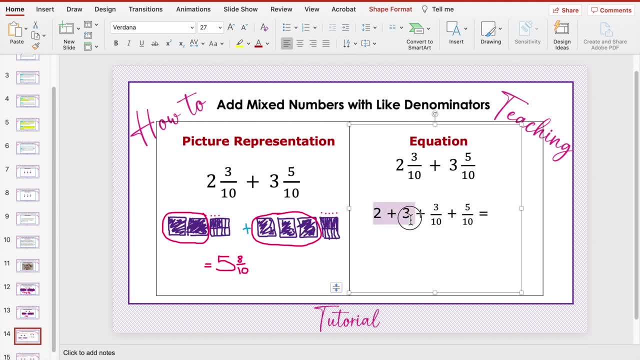 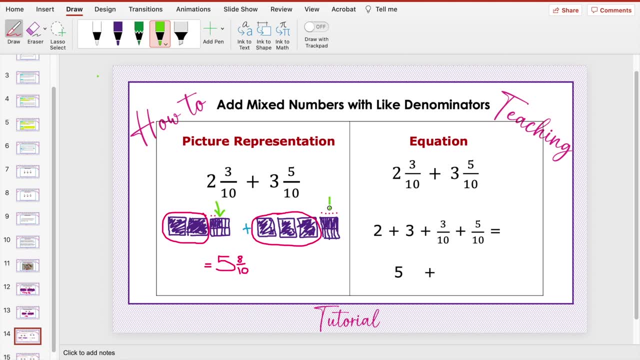 plus five 10ths. Then add the holes together to get a sum of five With the fractions. show students how the model of three 10ths and five 10ths is written in the equation. Also explain that we know the parts are the same size.